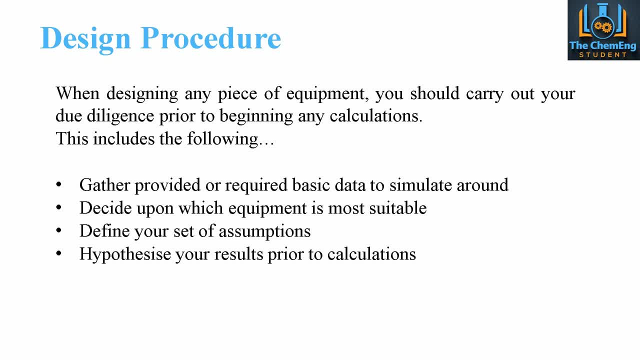 fixed beds, So we need to work out which one of these is the most suitable for our system. We then have to define our set of assumptions- and this is a really, really important step when we come to model- And then we have to have a hypothesis of what we expect the results to be. 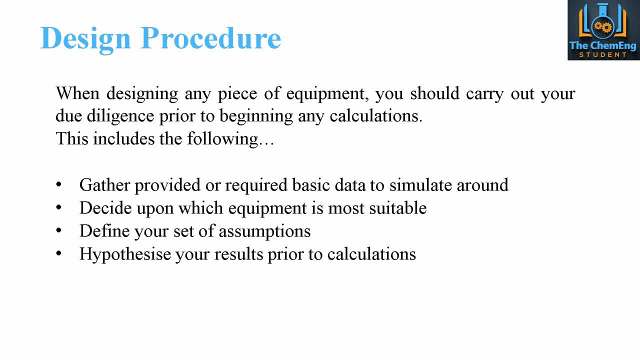 Now, of course, when you're designing a piece of equipment, your hypothesis is that it's going to work, but you could also have some ideas on your head as to how we could maybe optimize the system. Now, the assumptions are probably one of the most important parts, and we're going to have a look at some of the assumptions that we're going to make. 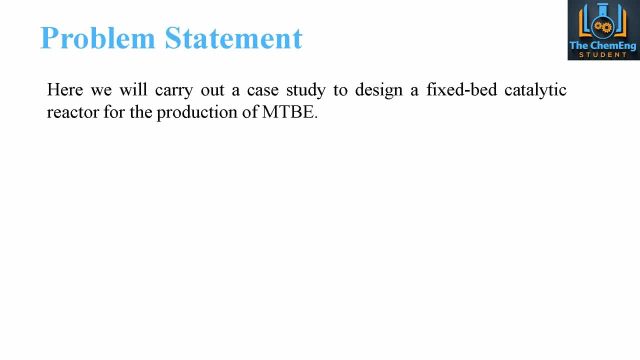 in this case study. Now, the problem statement is: we want to design a fixed bed catalytic reactor for the production of MTBE. Now, MTBE is methyl tertiary butyl ether, So normally produced through steam cracking. but here we're going to use a. 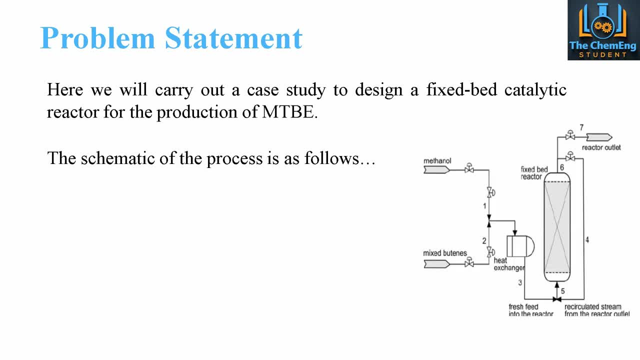 different process. Now the schematic that we're going to use here is something like this: Now this is taken from a real case data. Now we're not interested in the control scheme at this point, but we will have subsequent videos on how to create and produce control schemes. but here all we're really interested in is 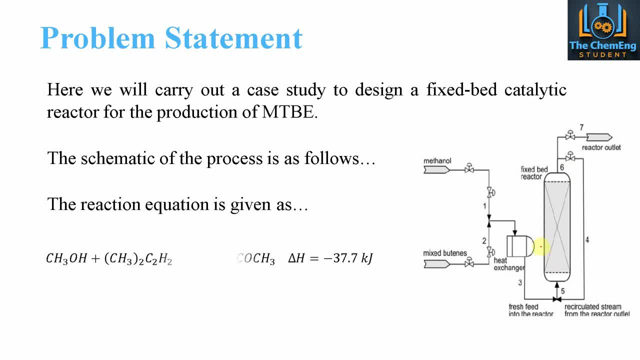 the generic fixed bed reactor. Now the reaction equation for MTBE is given by this expression here and we're given the delta-h value of minus 37.7 kilojoules. so here we have an exothermic reaction. Now we must carry out and 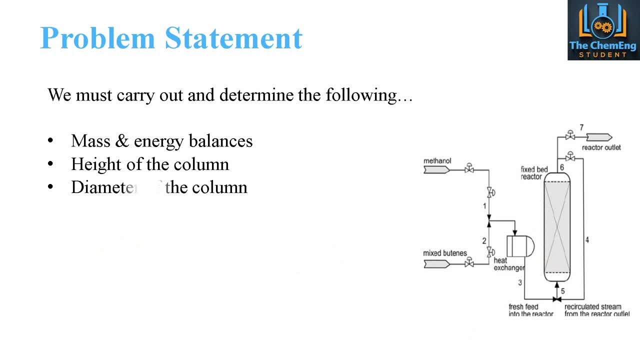 determine the following parameters: We need to work out the mass and energy balances around system, the height of the column, the diameter of the column. We need to work out the theoretical resistance time- sorry, resonance time, no resistance- the amount of heat generated within the system and we need to produce a schematic for the overall proposed design. 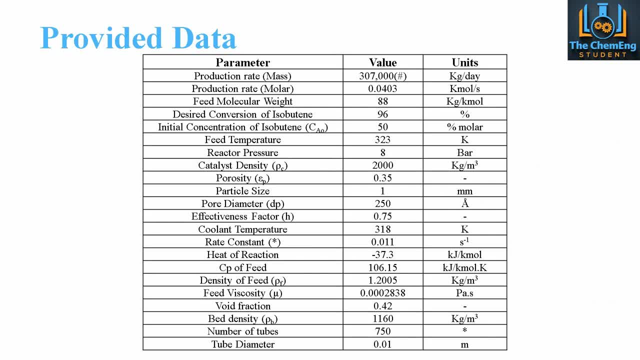 Now the information. as part of the due diligence, we have been provided with all of this information. So some of these values we will use, not all of them, but some of these values we will use in this part of the design phase. There are, of course, other parts of the design phase whereby we may take into account the effect of, say, the fluidization for the catalyst particles. 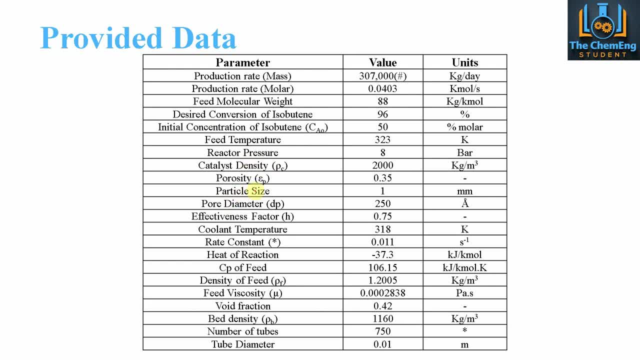 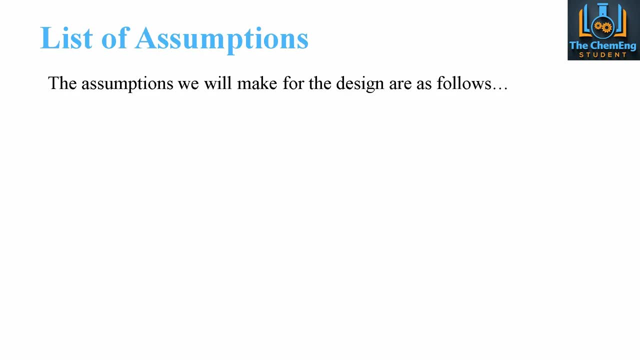 That's where the catalyst densities would come in, the porosity, particle size, etc. But here we're just going to look at the design process For the actual unit itself. Now, the assumptions that we're going to make here: there is a few, but we'll break them down into one individually. 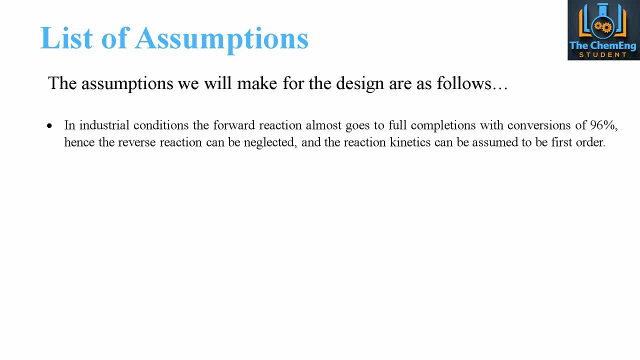 Now, the first one is that, for the industrial conditions, we're going to assume that the forward reaction goes almost to completion, Ie we're going to have a 96% conversion rate Now. the reverse reaction, therefore, can be neglegated from. 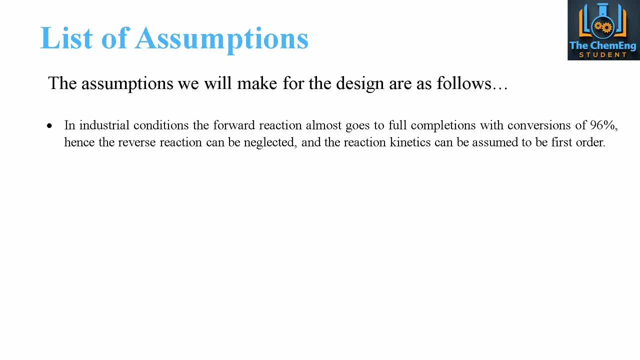 The system, ie we can assume that the reaction kinetics will be first order, because if we have a 96% conversion in the forward reaction and only 4% in the reverse reaction, potentially then we can say that the reverse is very, very small in comparison to the forward reaction. 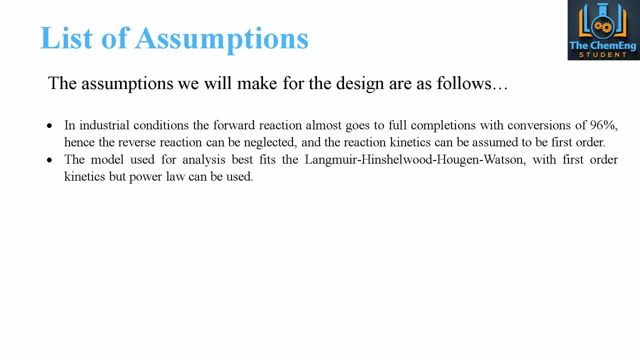 Now the model that we can use for analysis would best fit the Lagmuir Watson model. Now, this is what, of course, first order: kinetics, but here what we're going to use is the power law model. Now, the reactor can be assumed as adiabatic and under steady state conditions, so therefore we will neglect the accumulation term within the reactor, because what we're saying is what goes in per unit time is the same as what leaves per unit time. 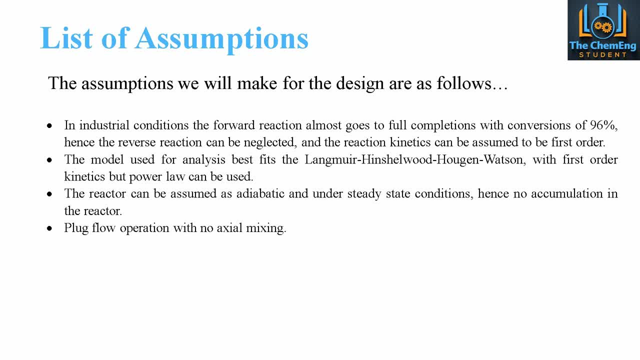 Now we're going to assume that we have plug flow operation with no axial mixing, so that's very, very important in order for us to determine what our base mass and energy balance equations are going to look like. We can then say that we have pseudo homogeneous conditions for the fluid and the solid interactions, so that's between the fluid and the solid catalyst. 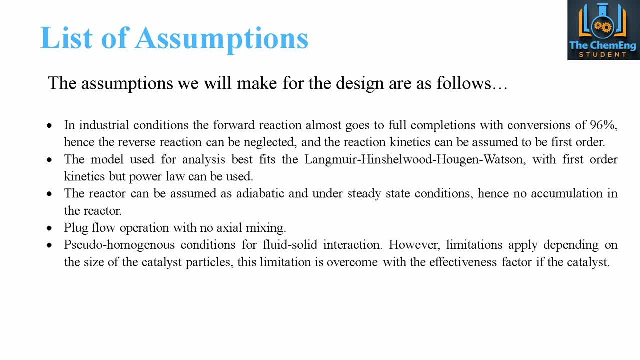 Now, there are limitations, though, depending on the size of the catalyst particles, but this can be overcome if we look at the effectiveness factor within the catalyst itself. Now, the main drivers of the reaction are concentration and temperature difference, because these play a significant role when modeling the reactor. 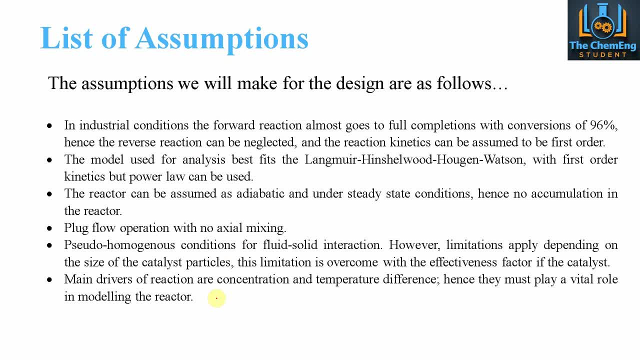 So that's what we're going to use as part of the mass and energy balances, And then, finally, that the pressure drop can be expressed using the Ergun equation if required, but in this case, for this case study, we aren't going to be concerned about the pressure drop, but we do go into the details in some of our online courses. 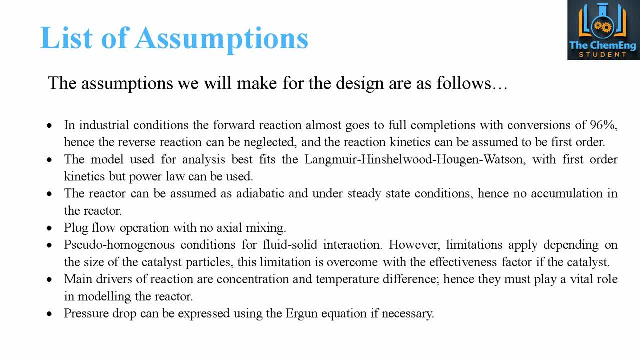 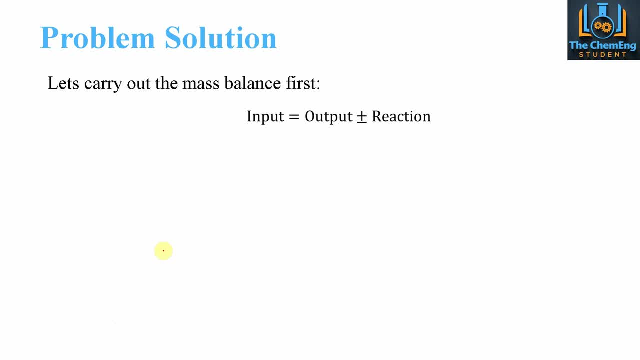 That concern problems with pressure drop. so I'll be sure to put a link in the description to those courses. Now let's take a look at the beginning of the solutions to this, because it can be quite extensive. but we'll start off by doing the mass balances. 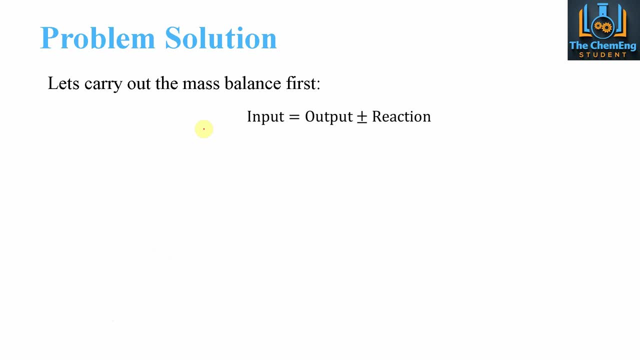 So we know that under steady state conditions we have the input must be equal to the output, plus or minus any reaction that occurs. So this is done for plug flow. So if we take, when we model plug flow now, we do it go into extensive detail in our reactor design course. 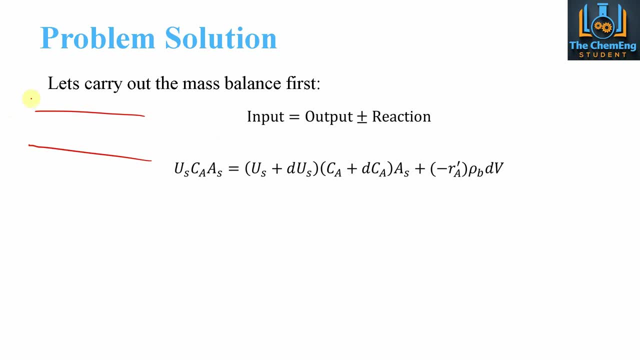 This goes into all the details that you would ever need to model every type of reactor, But here we'll just quickly summarize that when we have plug flow reactors- so this would be our in and this would be our out- When we model plug flow, we take a section and we model around this differential part. 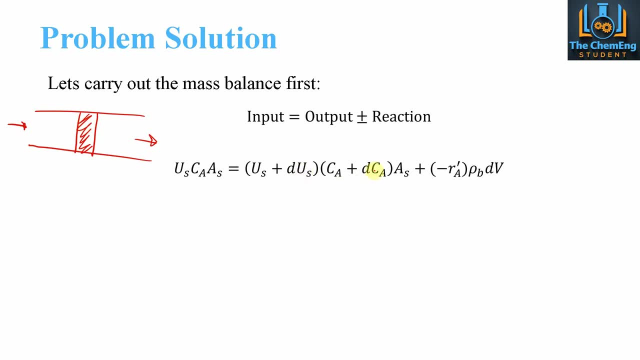 So this is where the DUS and the DUS are And this is where the DCA come from, because what we are measuring here is: US is the velocity, and CA is the concentration and A is the area. So that's the cross-sectional area of the system. 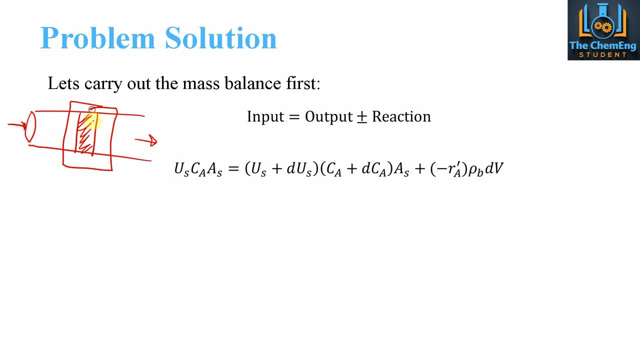 So this model is only applicable to this small chunk, But then we can scale it up to relate it to the entire reactor itself. So here what we're saying is the input coming into the system is going to be some velocity with a certain concentration. 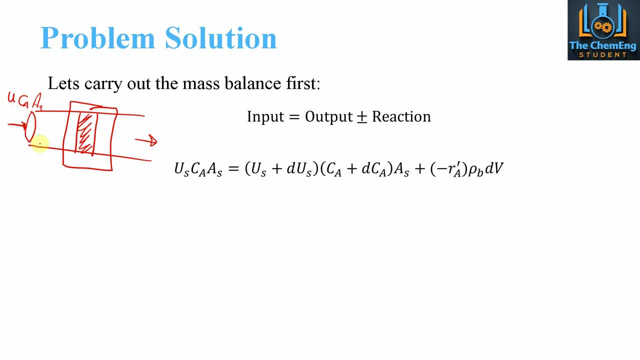 And the amount of velocity and the amount of concentration can be represented down in a surface area. Now, granted, the surface area isn't going to change. So that's why AS isn't a differential function, because AS is going to remain the same. 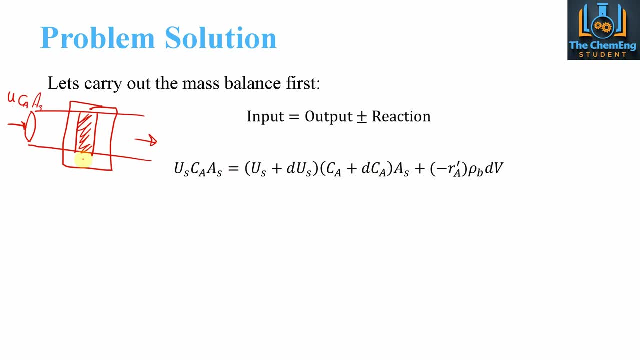 Now, when we surpass this point in time, we will then have picked up or last a amount of velocity and an amount of concentration. So that's where we have our velocity plus the velocity plus the concentration. That's different. that accounts for this section. so that's the DUS, then multiplied by CA, so that's. 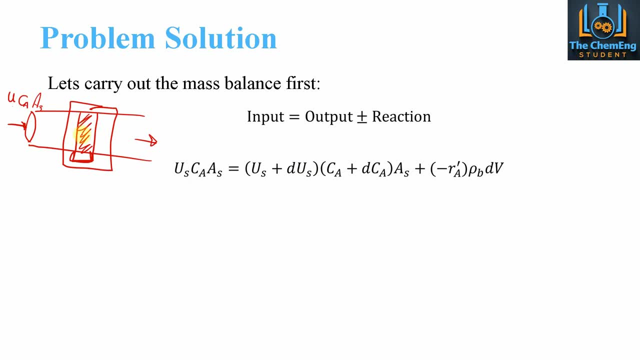 this CA plus the part that we've picked up or lost in this section, multiplied by AS, and that's going to be equal to the reaction, which is the rate. so minus RA is the rate of the reaction multiplied by the density, multiplied by the change in the volume. so 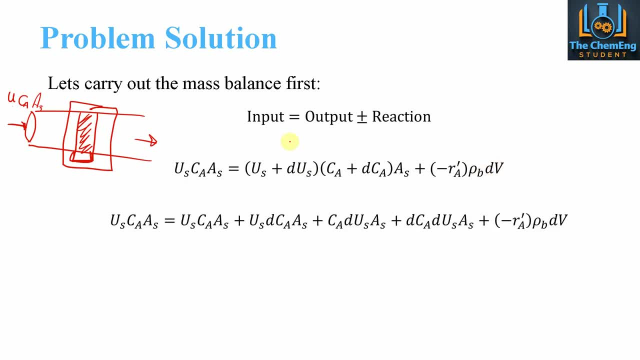 that's the DV. So now what we can do is expand these brackets like so and remember to account for the AS in each of the multiplications. So here what we can see is that we end up with some similar terms. So right away we could cancel this term and this term so that 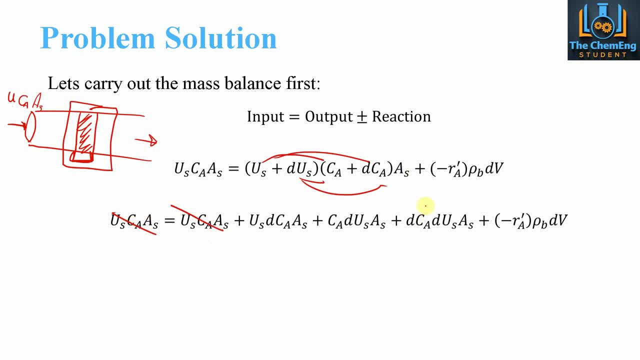 makes the remainder equal 0.. Now, another trick to this, when we model plug flow reactors, is that you will always get a term whereby we have the DUS. Now, this term is very, very small compared to the other three terms. So what we can do: 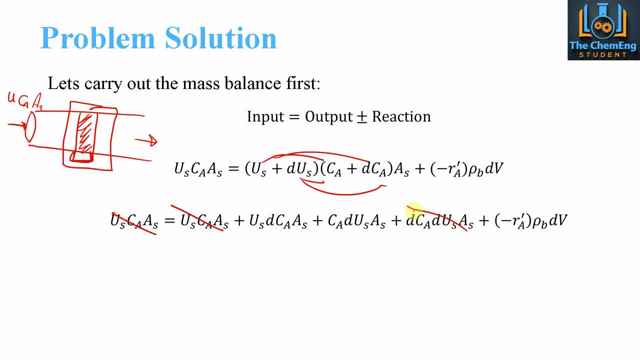 is. we can actually mitigate this because it is incredibly small in comparison, so the influence isn't that great. So what this allows us to do is simplify the equation even further. Now we're almost there, but we now need to simplify the equation even further, So we 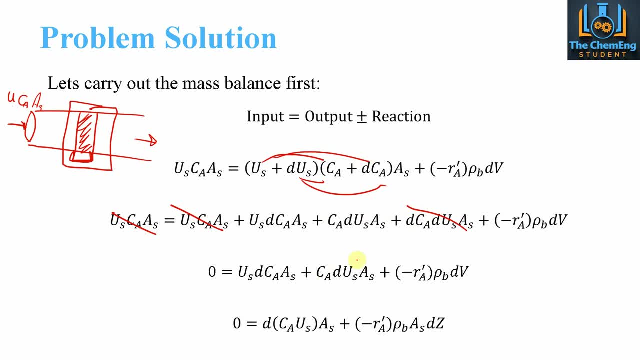 can do that. So we have a simple, easy way to start to collect some of these like terms, And what we can do is we know that the DCA and DUS are both functions of the area, So we can group these two systems together And what we find is that we have D, so a function. 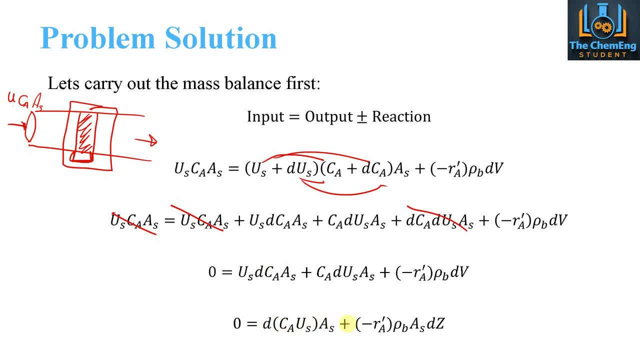 of CA and US multiplied by the area Plus, then we have a reaction rate multiplied by the density. but this time we need a function of CA and US. So what we can do is we can in terms of the height. so we then have to change the volume, so dv, because dv is the change in the 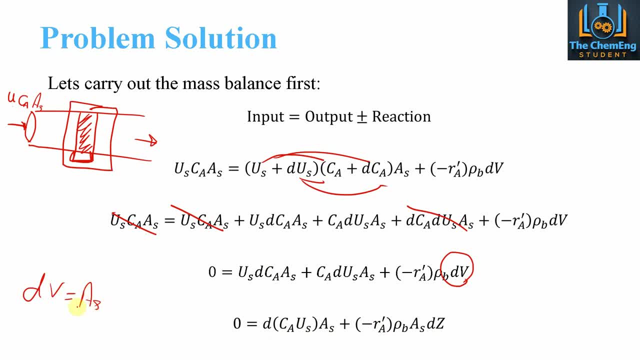 volume. so that's going to be equal to the area. so the surface area multiplied by the height and the height is z. but remember, as we move from here along to here, the height value is going to change. so that's why it is dz and not a constant z, because a is going to remain constant throughout. 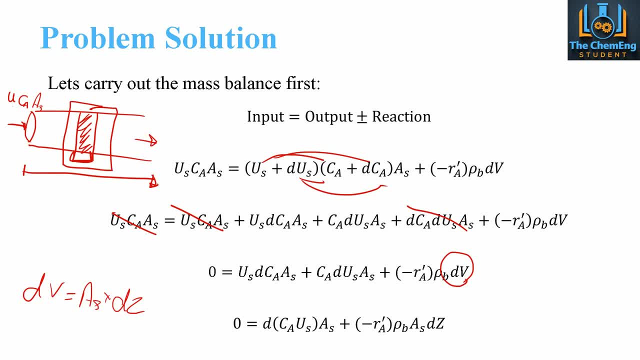 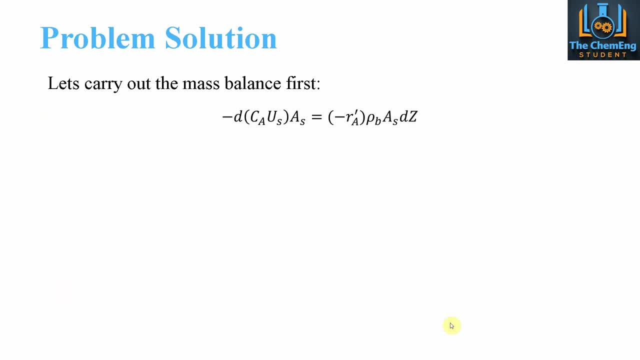 the surface area at any given point in time is going to be the same. so that has now got as a function of the height, and that's what we need. so then what we can do is bring the second equation across to the other side, and then we can start to separate these out. we can bring the dz across to 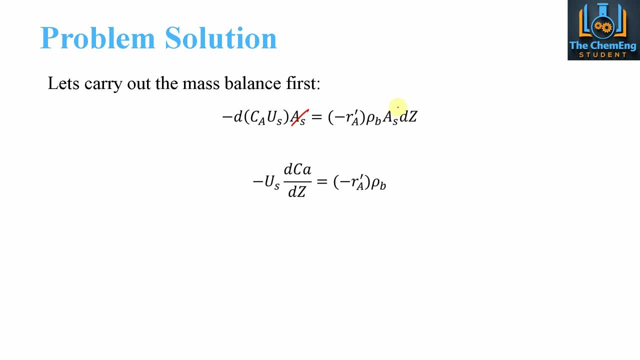 the other side, and what we can do is we can cancel out the surface areas on both sides of the equation. and what we can do is we can cancel out the surface areas on both sides of the equation, and what we can do is we can cancel out the surface areas on both sides of the equation. 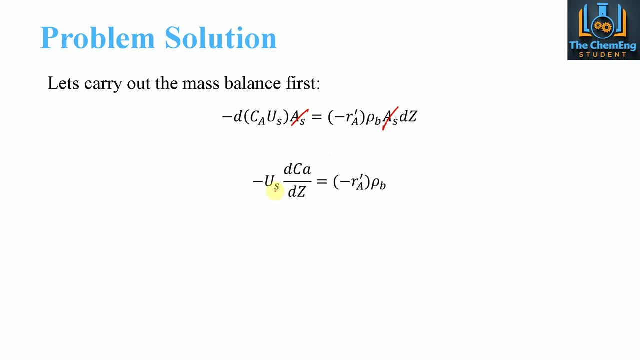 what we can then be left with is minus the velocity multiplied by the ratio between the change in the concentration and the change in the height, because we're taking the velocity as constant, ie we have steady state conditions- and that's equal to the reaction rate multiplied by. 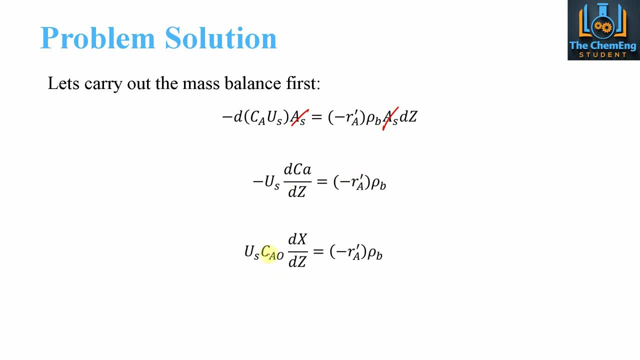 the density. so then, finally, what we can do is we need this in terms of conversion because, as it stands just now, ca is the final concentration. now we don't know any information about the concentration as of yet, but what we do want to know is what the height is going to be. 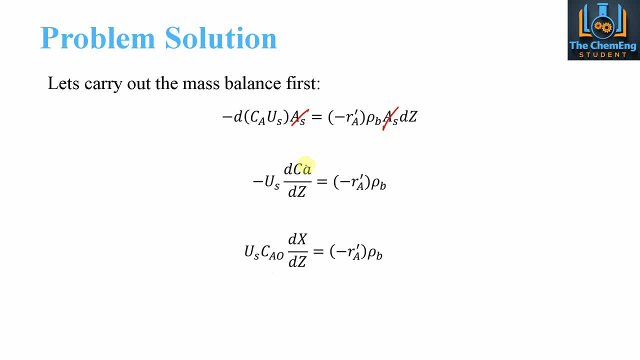 at a given conversion, and we know our conversion is 96. so what we have to do here is change the dca as a function of x, and the relationship that we exploit is that ca is equal to ca naught one minus x. so that's the relationship that we exploit. 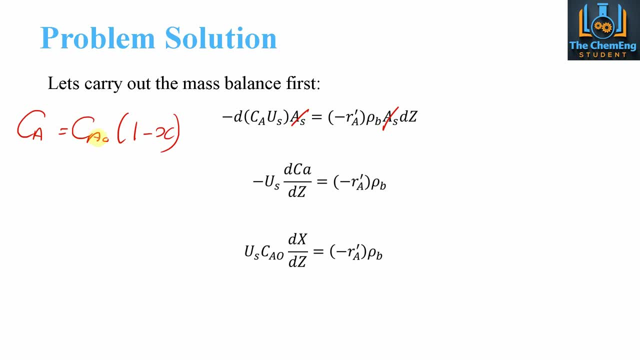 that's where the initial concentration is going to remain constant. so therefore we bring that out and that multiplies the, the velocity. but in doing this we can see that we would end up with a negative c, a naught. so that's where this negative is then removed, and then we have a change. 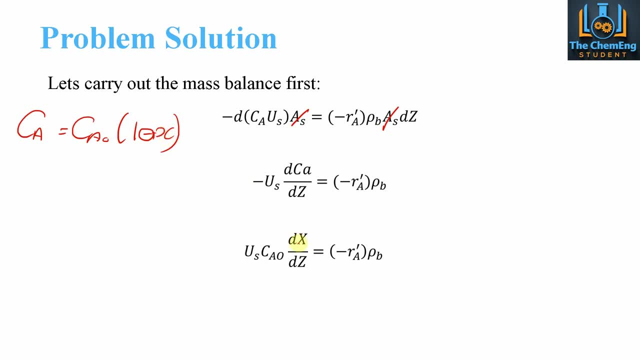 in the constant a, sorry, the change in the conversion. so that's why we have dx by dz, so we can then bring these constants across to the other side and we can see that our relationship between the conversion and the height is given by minus RA multiplied by the density, divided by the velocity, multiplied by the initial concentration of A, And that's. 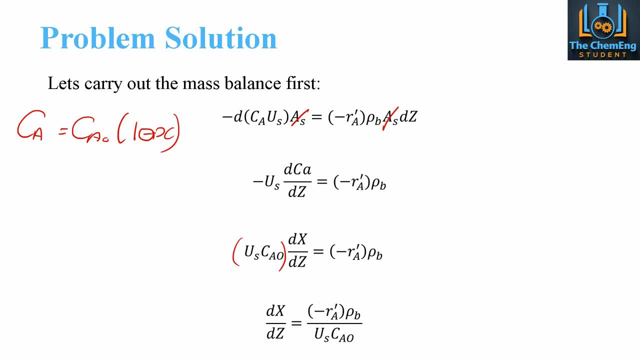 the mass balance done for this system, Then what we can do is now we can turn our attention to the energy balance. Now the energy balance is we have accumulation is equal to the enthalpy in minus the enthalpy out, plus or minus the heat of the reaction, plus or minus the heat. 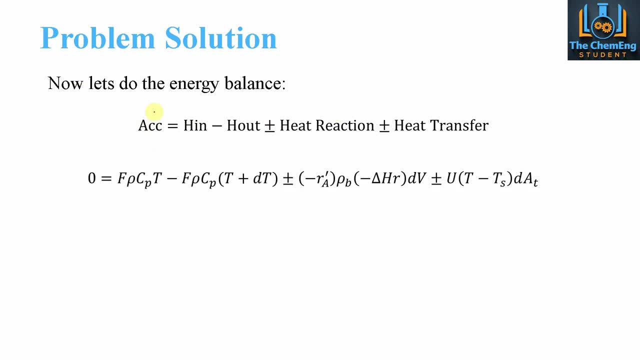 transfer. So what we can then do is we, because we said we had steady state conditions, we can assume the accumulation is zero. Now F here is the flow rate of the system, but we can also denote this as Q as well, So we have the flow rates coming in for both of these. 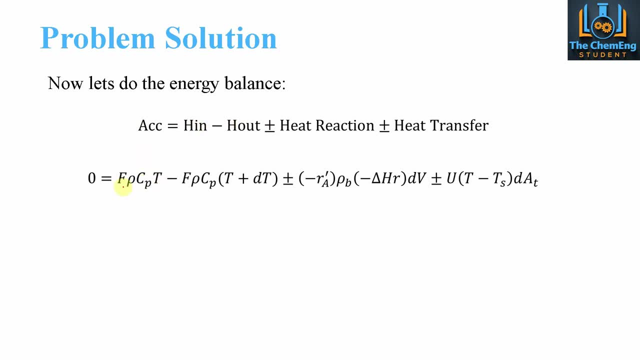 because, remember, this is a movement, it's not a batch reactor. So we have F multiplied by the density, Multiplied by the specific heat capacity of the fluid, Multiplied by the given temperature. Now, again, just like when we did with the concentration, we are modelling around this section. So we 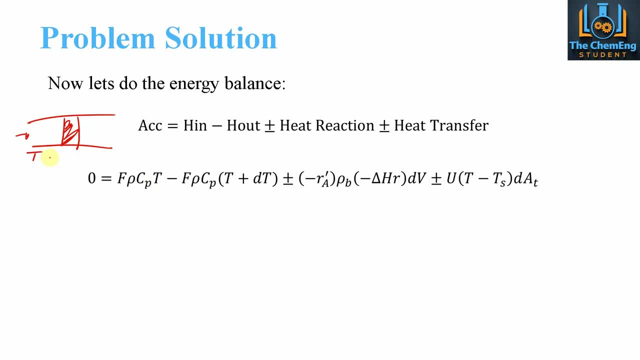 have T coming into the system some point temperature. We then pick up or lose temperature, So this would be the DT. So then the output here would be T plus Whatever the value of DT is. Then we have our heat of reaction. so that's the reaction. 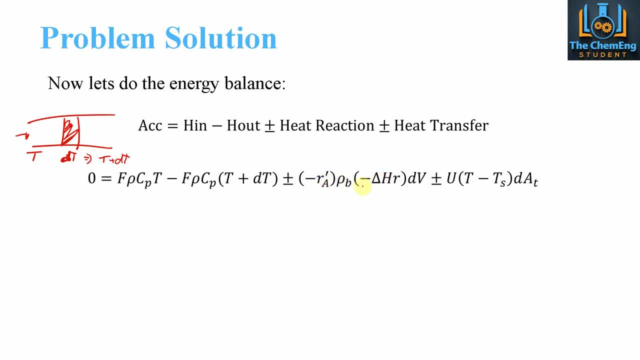 rate, multiplied by the density, multiplied by the heat of reaction, so that's minus Delta HR multiplied by the change in the volume, because, remember, this will of course change as the volume changes, and the volume will allow us to convert from back into the area and then back into the height as well, if we want. 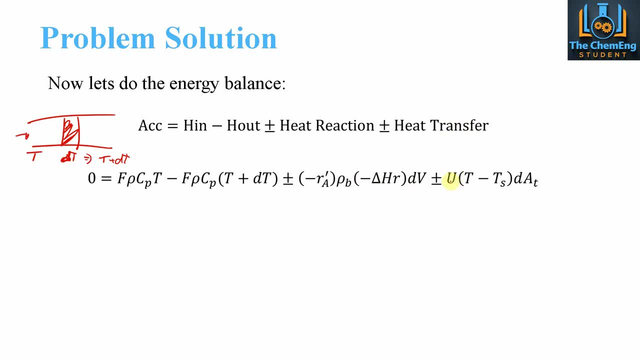 and then the heat transfer is just going to be the U, so that's the overall heat transfer coefficient multiplied by delta T, which in this case is going to be T minus TS. so that would be T and TS multiplied by DAT. now, lowercase T is the residence time. 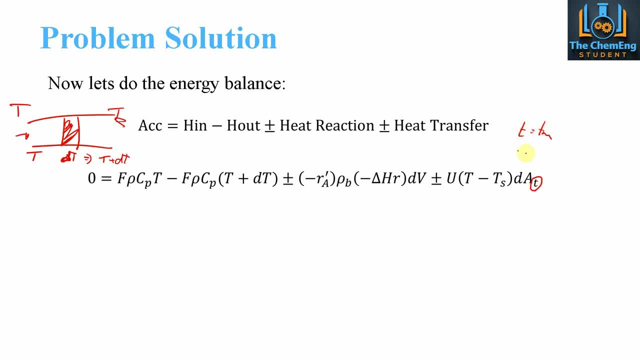 so lowercase T is time and capital T is the temperature. so that's the major distinction. now what we can do is we can bring this term across and that will go over as plus. so that's all we've done here. then what we can do is we can say to ourselves: 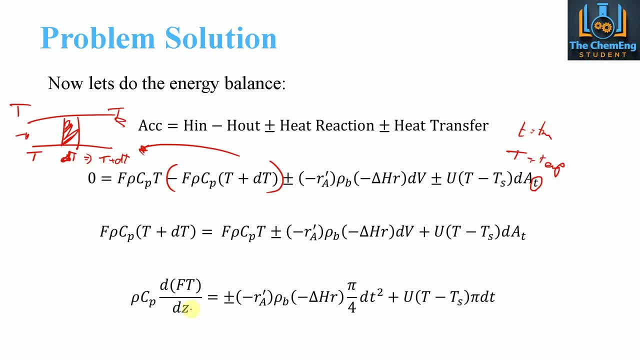 we can cancel out, or attempt to now cancel out some of these terms and in doing so we can see that the F? rho CPT and F? rho CPT that is going to cancel. so here we end up with that: the rho CP is multiplied and we have a differential of the flow rate and the temperature. 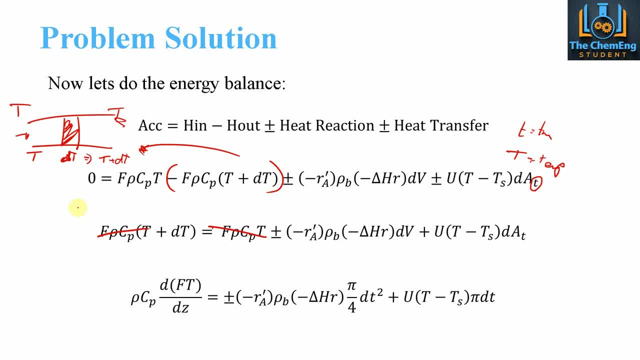 with respect to the length or the height of the column, and this is equal to minus RA, rho B multiplied by heat of reaction, minus delta HR. and then this time we have the cross sectional area, because we've turned the DV into the area multiplied by the height. 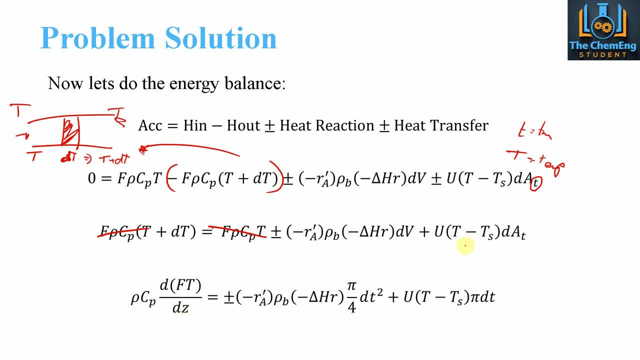 so that's how we manage to get the DZ across the column. so then what we then have is we have our pi over 4 D T squared, and then we have now replaced the DAT with pi D T, because we replace the area with this parameter. 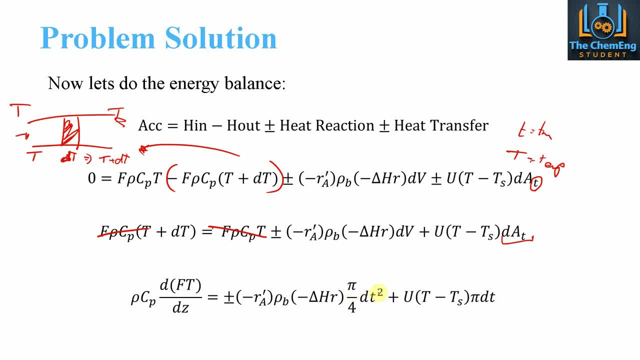 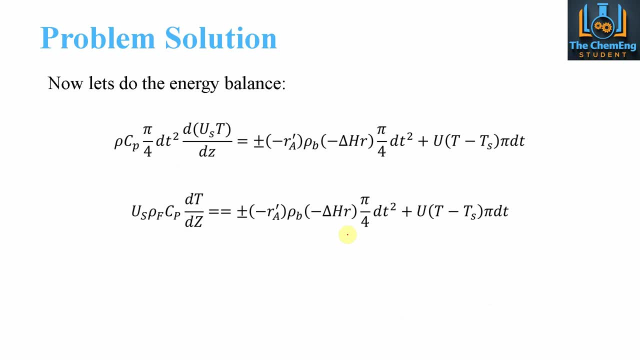 and that will give us a cross sectional area as a function of T, and then we can then start to simplify this again. so what we end up with is now we can rewrite this: if we bring the pi over 4, we get that across to the other side. 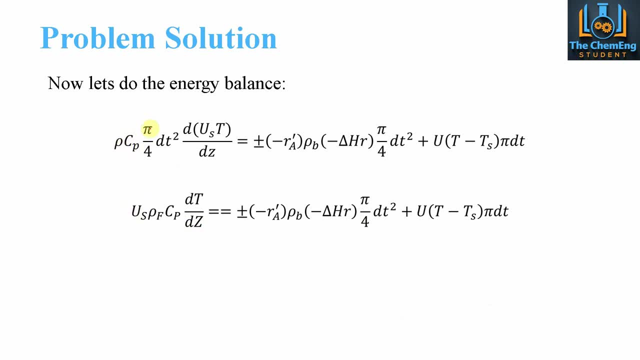 then what we can end up with is rho CP, pi over 4 D T squared. we can then replace that as U rho CP. then that would be D T over D Z, because we are assuming here that the velocity is going to be constant. and then what we can then do? 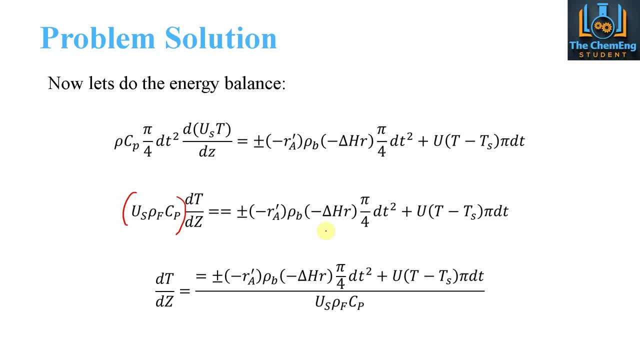 is divide by this term on all of this equation and we get the relationship between the change in the temperature with respect to the change in the height. so that is the energy balance for this system. so we've answered the first part of the problem statement. now the second part. 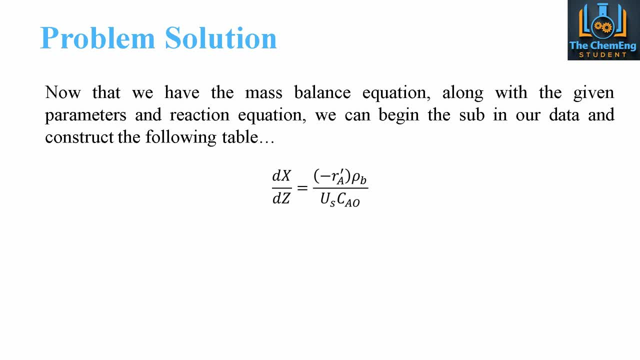 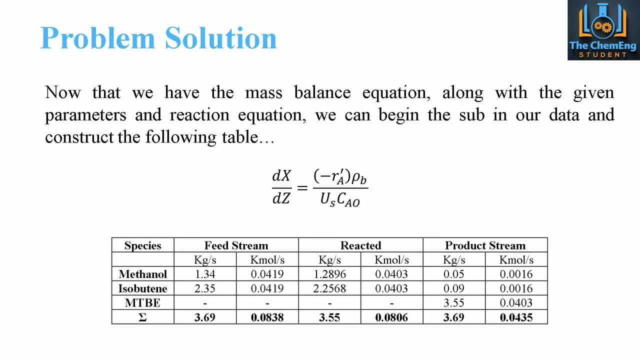 is that now we have the mass balance, we can then begin to substitute in our data and we can therefore create this table here. so this is, as worked out, the composition in terms of kilograms per second and kilomoles of the feed stream, the amount of feed stream. 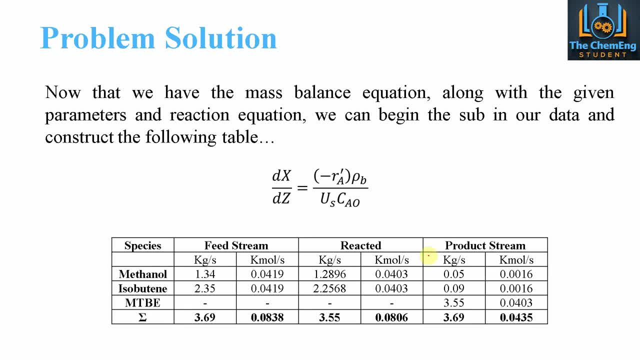 the amount that is reacted and the outlet product stream. and we've done this by using this equation, because here what we would have is we would have: D X is equal to. it would be minus R A, prime rho B over U S C A naught D Z. 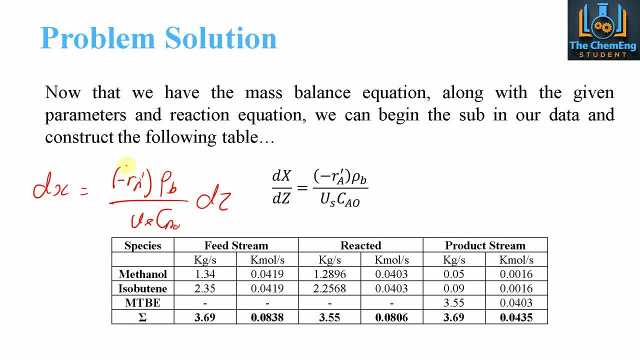 so we could then change the values for the conversions and work out. this is just standard mass balances. now, if you're unsure as to how to get these values, be sure to check out our mass and energy balance course. I'll put a link in the description to that. 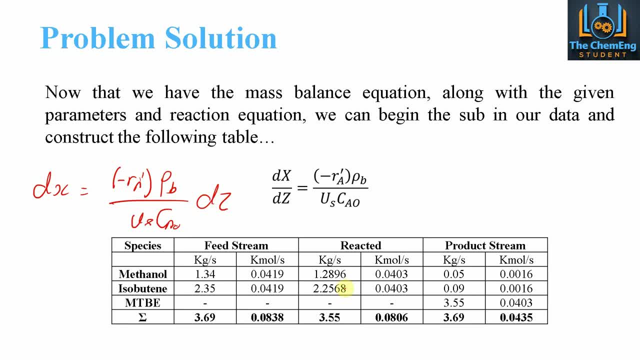 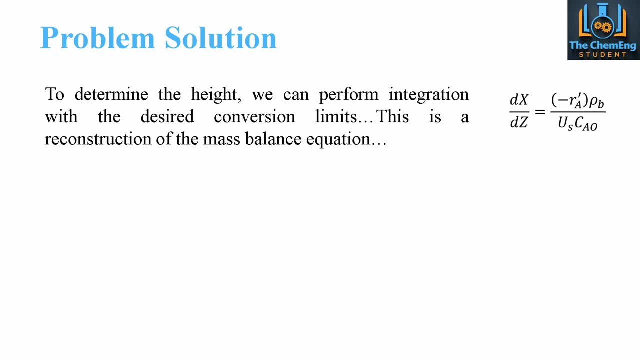 and you can have a look and see how easy it is. in order to find these values, we just use a basic species table. so now, what we can then do is we can now start to determine the height, because what we can do is perform the integration with the desired conversion limits. 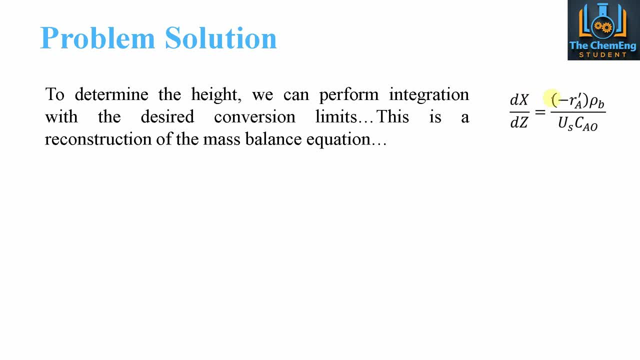 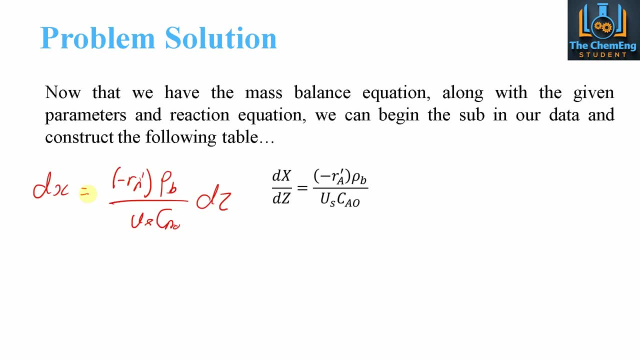 and this will then allow us to reconstruct the mass balance equation. so we go from this to this. now, the way that we've done that is very similar to how I wrote it here- is that we've split this apart and we've got rid, so we've got the D X and the D Z. 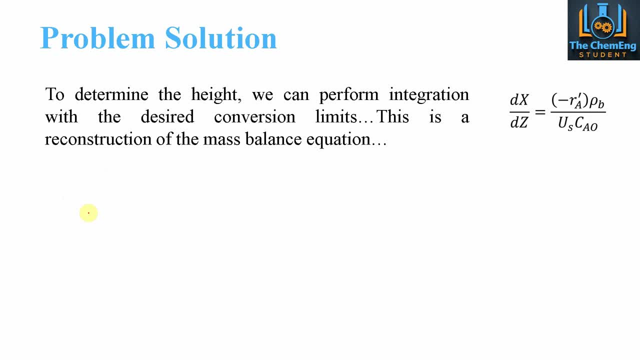 as individual functions that we can therefore start to integrate now. in doing so, we know the limits of our conversions. we know it's between 0 and 96 percent, ie 0.96. now what we want is this: unknown here, Z, because we know that at 0.0. 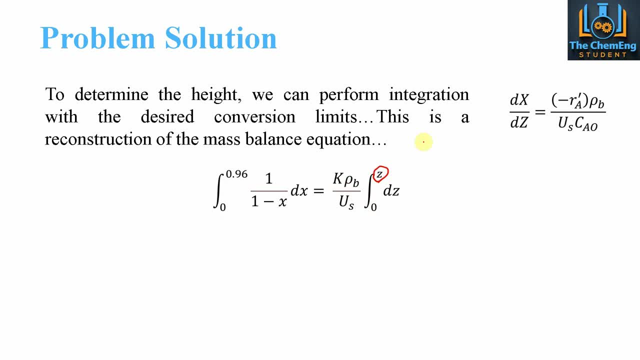 for the conversion. our height is going to be 0. now what we have here is we have this new K and we've got this strange function here. now what that is? that's because we've rewritten the rate expression, so we've done minus R. A is equal to K, C, A. 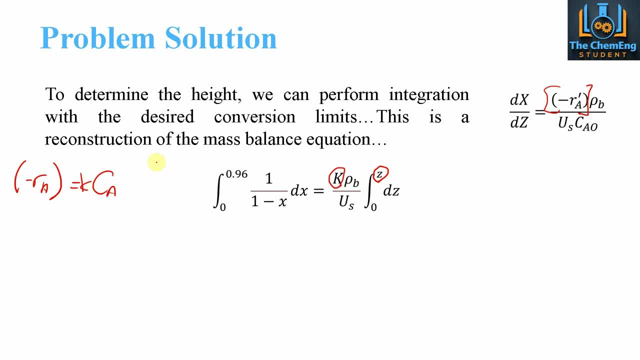 that is your first order reaction rate. so that K. there is this K. so what we've then done is we've brought the K from here. sorry, we've brought the C A across to here, so this thing goes over as 1 over C A. now we need it in terms of conversion. 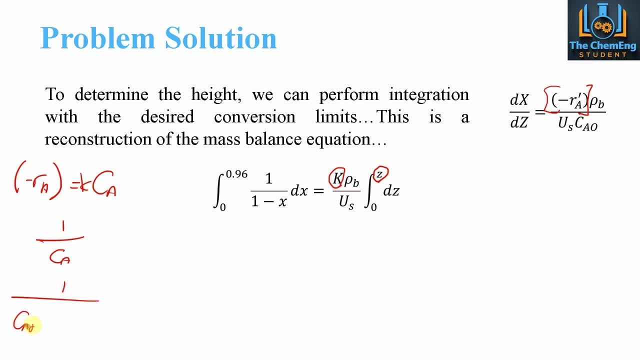 so we have the 1 over C A naught, 1 minus X. now when we solve, we end up with this equation here, and that is just the function of X, and that's exactly what we need, because we are differentiating with respect to X. so now what we do is we substitute in our values. 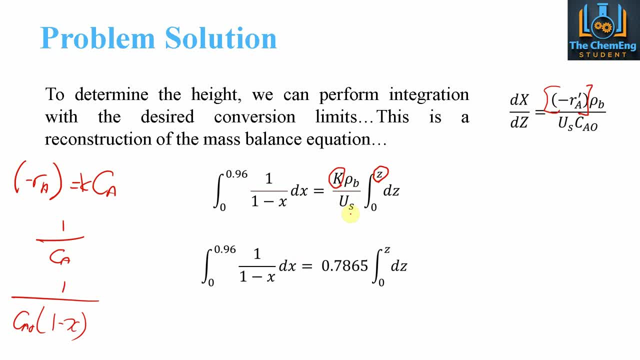 we know all of these terms from the data that we were provided, so what we can then do is integrate this, so we get 0.7865 multiplied by Z, because this is 1, so when we substitute in the 0 and the Z, we get Z. 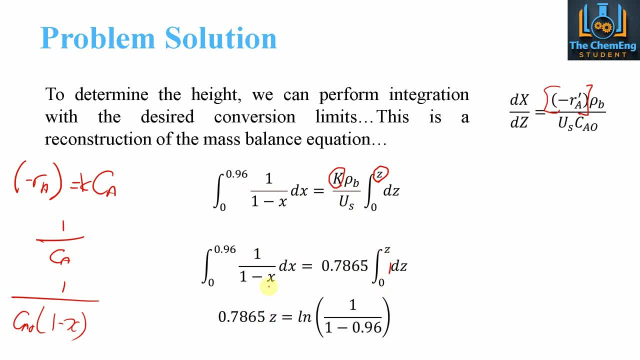 and then this will be a logarithmic function that we will get, because we have 1 over the function of X, so we get ln of 1 over 1 minus and then it will be 0.96. now we don't need to include the 0, because we would have ln of 0. 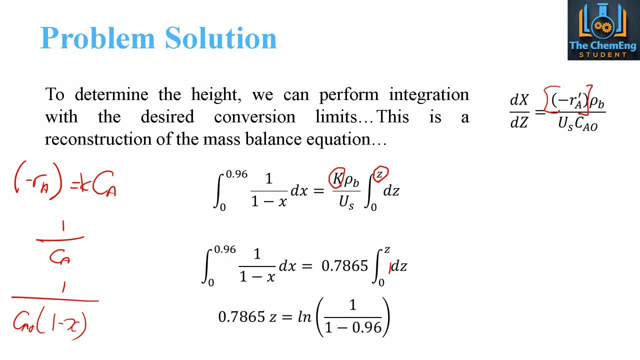 so we don't need to include that in the system now. we just divide by 0.7865, and that will tell us that the height of this column, when we design it, is 4.08 meters, and that's the height that we would need. 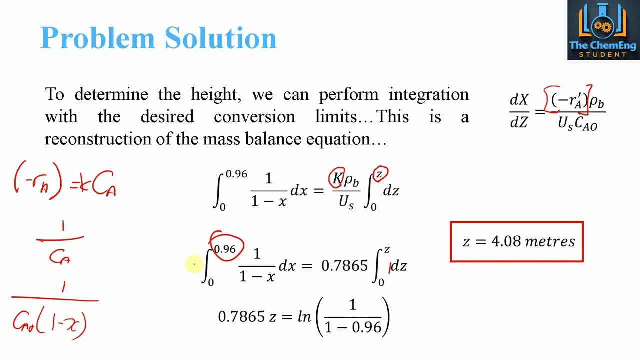 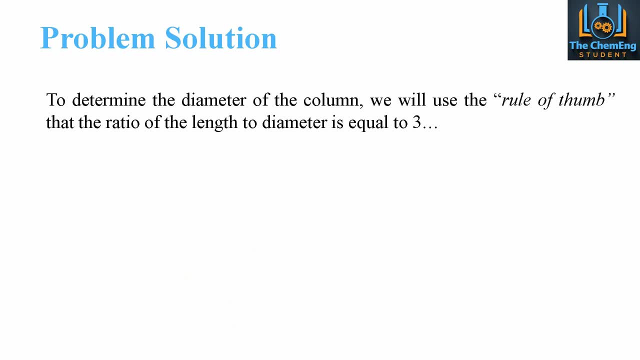 in order to achieve a 96% conversion. now, in order to determine the diameter, we use what is known as a rule of thumb. now, there are several different renditions of the rules of thumb, but here what we're saying is that the ratio to the length and diameter 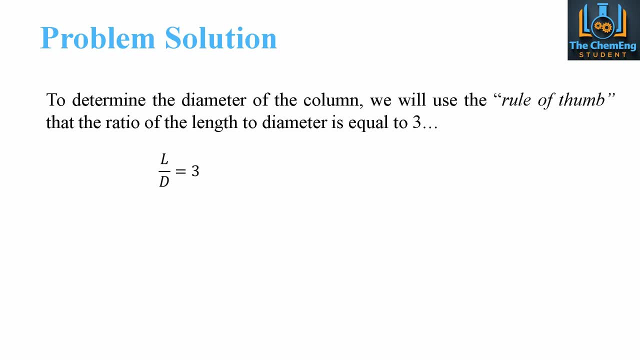 will be equal to 3, ie the diameter is 3 times that of the length. so therefore, what we can say is: we now know the length is 4.08. we substitute that in divided by 3, so we know our diameter is 1.36 meters. 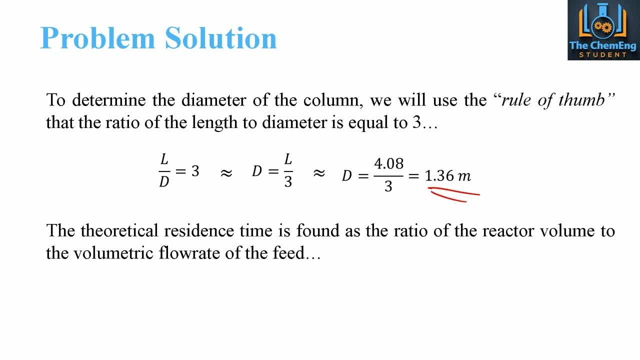 so very, very straightforward now. the theoretical residence time is found as the ratio of the room to the room, which is equal to the volume of the reactor, to the volumetric flow rate of the feed. now this is given as the greek letter, tau, so tau is equal to the volume. 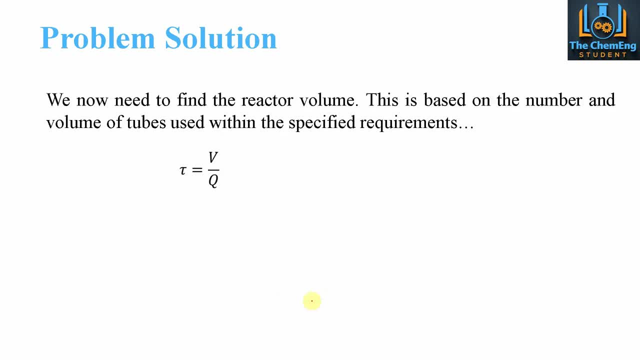 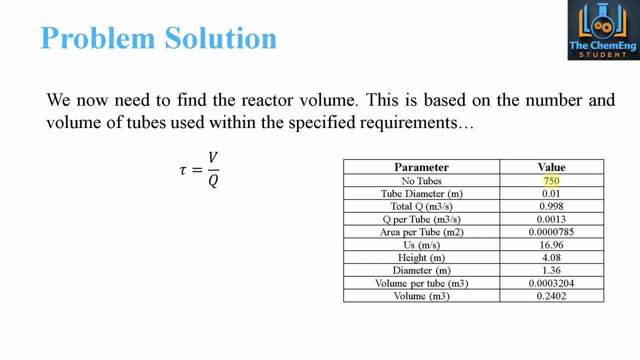 divided by the volumetric flow rate. now, what we then need to say is: this is now dependent on the number of tubes, and what we need to find is: we go back to the problem table, and that gave us information about the number of tubes, because we were told that we had 750. 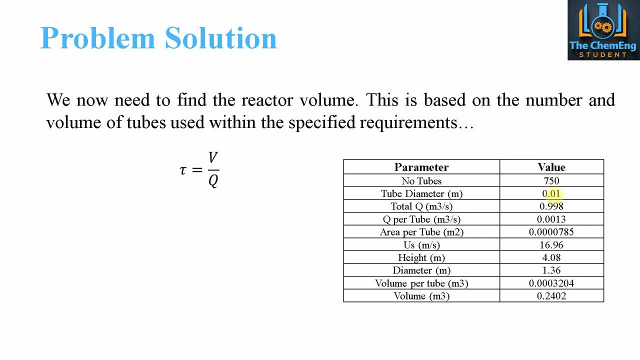 and we know the tube diameter was 0.01 meters. so what we can start to work out here is we can start to work out what the area is. so we know the area per tube will then be pi over 4 d squared, so it will be 0.0000785 meters squared. 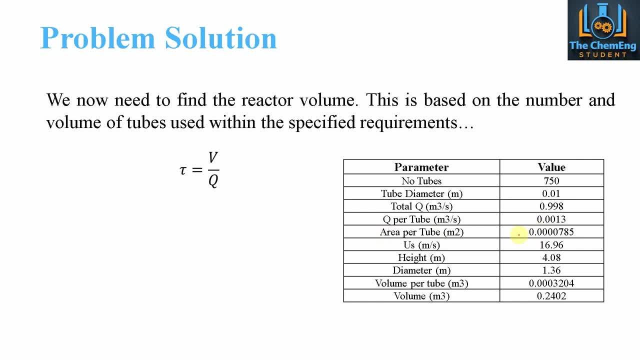 that's the area of one tube. then what we can do is we say that we can, so we could multiply this by the length and we could work out that the volumetric flow per tube will be equal to 0.0013 meters cubed per second. 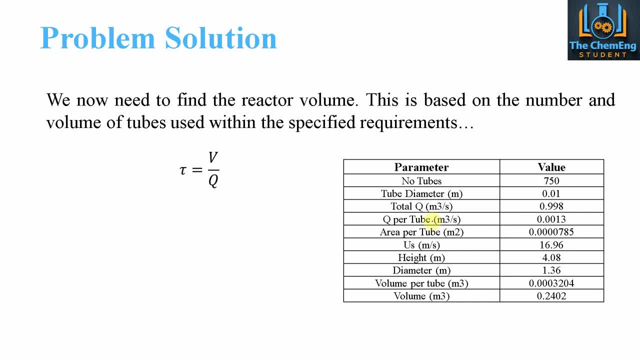 so that's the volumetric flow per tube. now the key thing here that we want is that we now need to know what the overall total volumetric flow is for the entire tubes. so we take this value and we multiply it by the number of tubes, and that will give us 0.998 meters cubed per second. 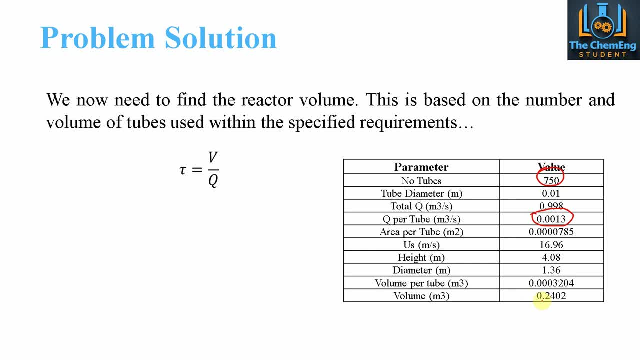 and we already know what the volume is. the volume is given as 0.2402 because we can work out the height or we work that out. we know the diameter, we can work out the volume per tube, we multiply it by 750 and that gives us our 0.2. 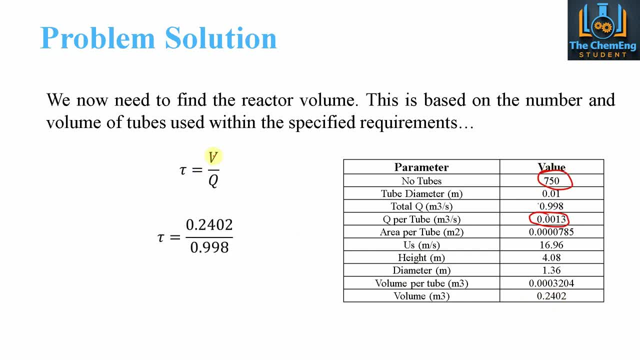 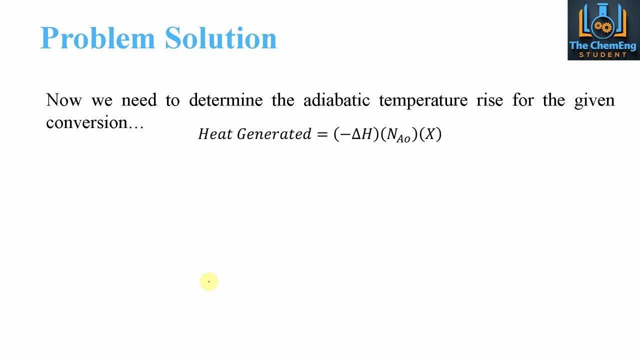 so what we can then see is that when we substitute in these values, we end up with: tau equals 0.2, 0.24 seconds, so it's an incredibly short theoretical residence time, and that's how you would go about finding the theoretical residence time. 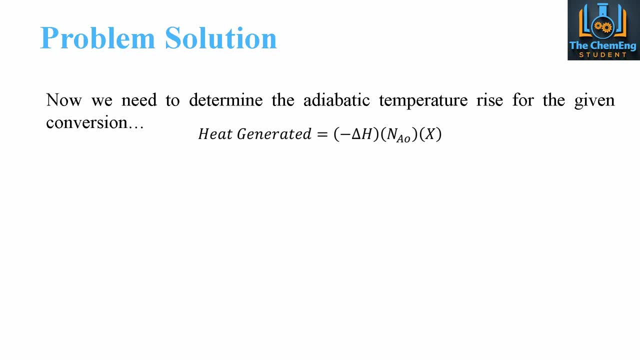 now. we now need to determine the adiabatic temperature rise for the given conversion. so what we need to do is work out that the amount of heat generated is equal to minus delta H multiplied by the initial number of moles multiplied by the conversion. so what we end up with is we: 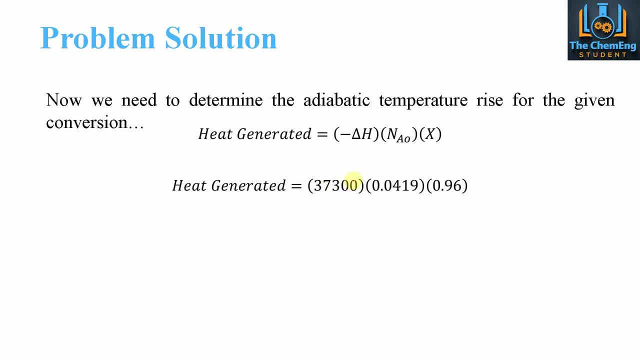 were given that it was 37,300 joules multiplied by the initial number of moles of A, which was given to us as 0.0419, multiplied by the conversion of 0.96, this tells us that the heat generated will be 1500 kilojoules per kilomole. 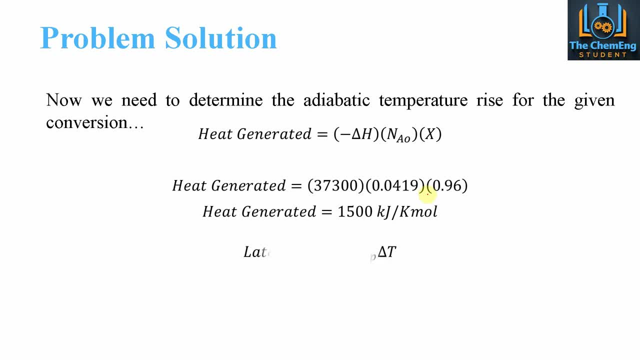 now, that is the latent heat within the system. so that will then allow us to determine delta T, because the latent heat is going to be the flow rate multiplied by the specific heat capacity, multiplied by the difference in temperature. so when we substitute in the values, we can work out that our delta T value. 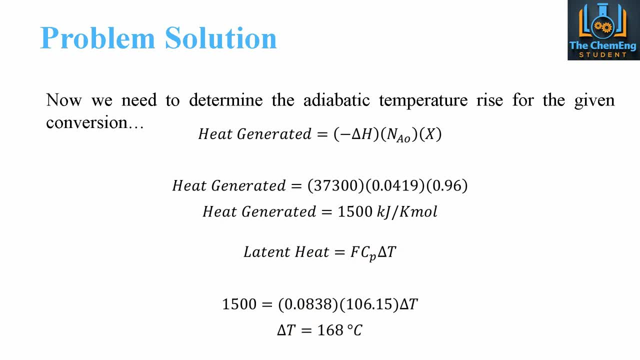 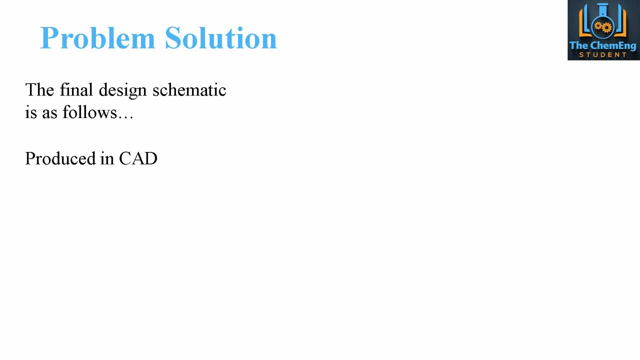 is going to be 168 degrees Celsius. so that's our adiabatic temperature rise for this given conversion. so now that we have found all the required parameters, what we would then do is take the mechanical dimensions, put it into CAD, and then we can design the reactor. 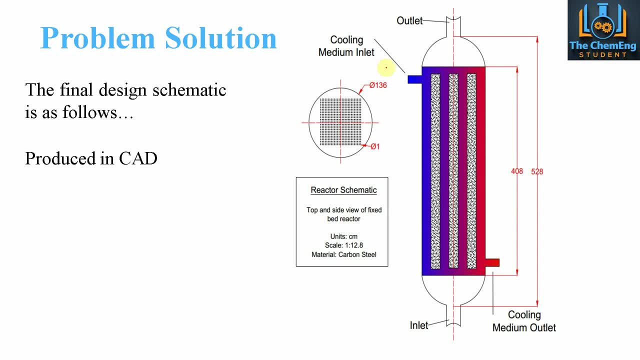 to look something like this, whereby we have our heating and cooling system within the reactor, so we can see that we have our inlet for our cooling and we have our outlet for our cooling stream, so we can see that it is heating up gradually as we go from this point to this point. 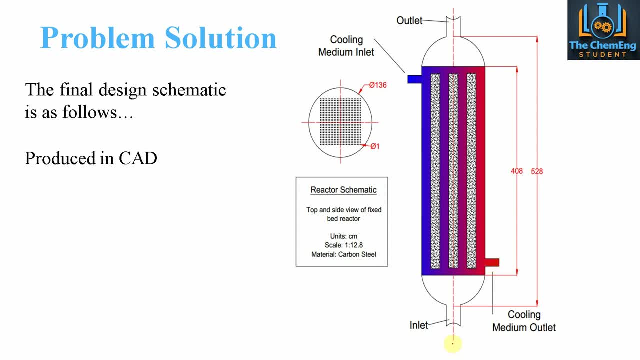 we have our inlet for our fluid and then we have our outlet that comes out the top, so we are getting that counter current flow. we have our height of the reactor bed, then we take into account the radius of the heads and the bottom, so therefore we get a total height of 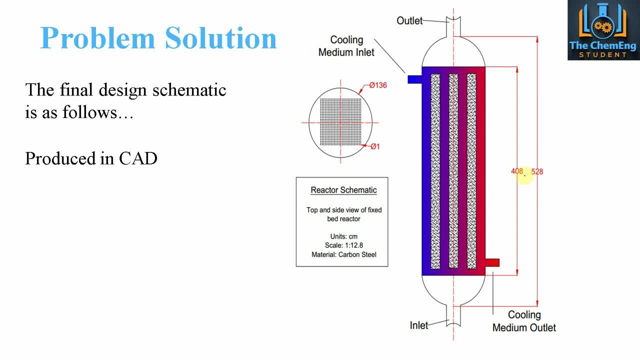 528 centimetres or 5.28 metres. now our scale here is given as 1 to 12.8. we are assuming a carbon steel material, and then this would be our cross section if we were to look down upon our system. so here there is 750 individual tubes. 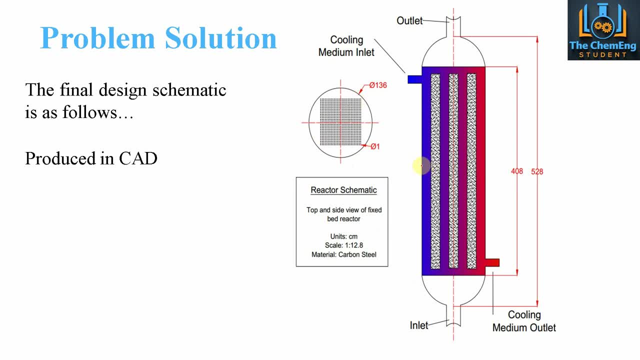 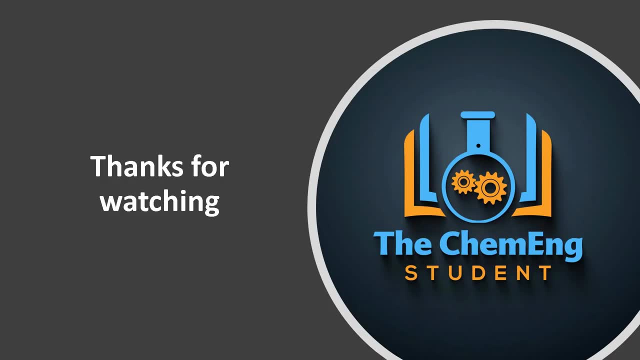 and that is what your cross section would look like and that is how you would go about solving a full catalytic fixed bed reactor. so that is the end of this lesson. thanks for watching. hopefully this was helpful in showing you the process on how to design and model.